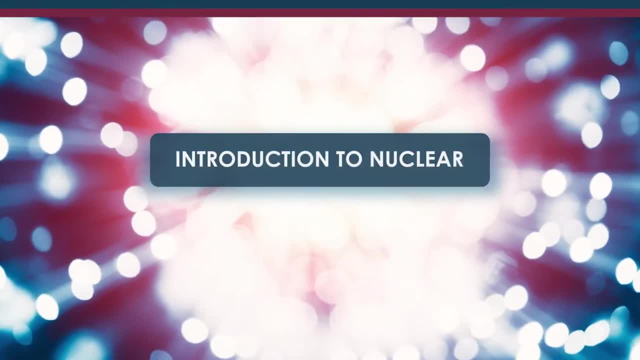 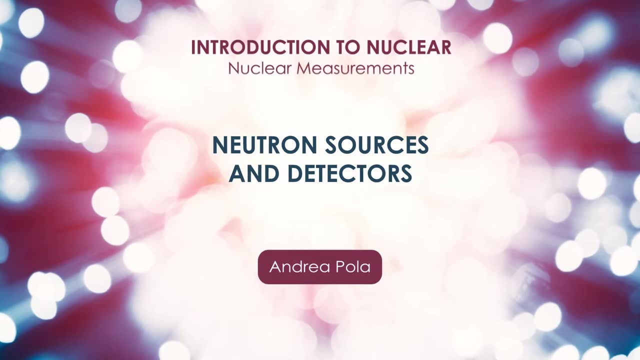 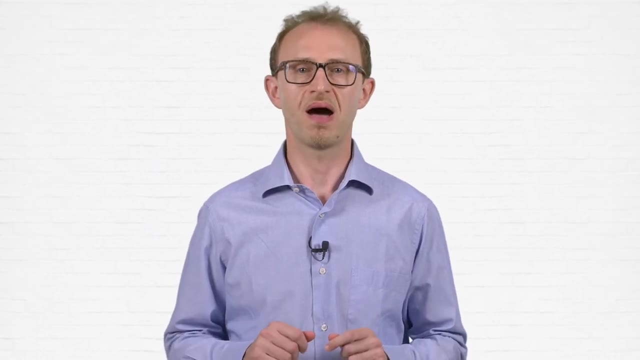 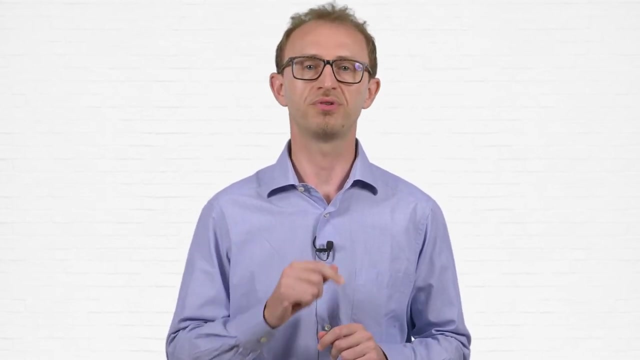 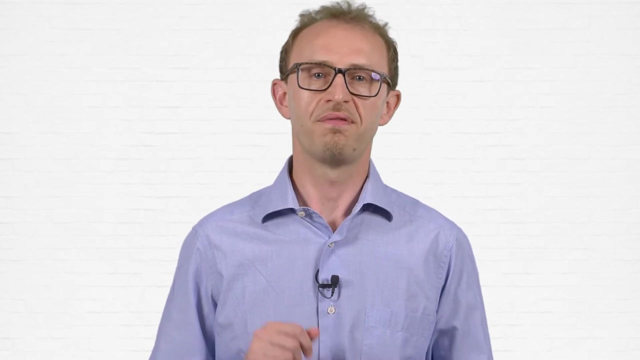 Neutrons are the neutral particles bound inside the atomic nucleus. We all agree about that. but do you know? they can come out of the nucleus, ejected by a decay process or by a nuclear reaction. Ok, follow this lecture. Here we'll present a quick overview of neutron sources and a 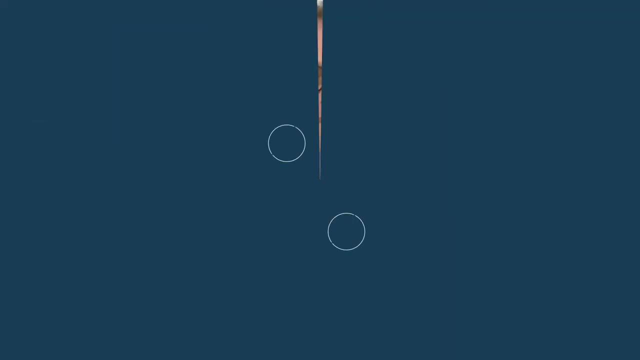 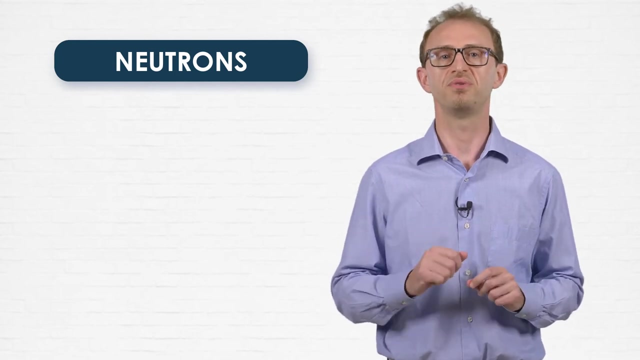 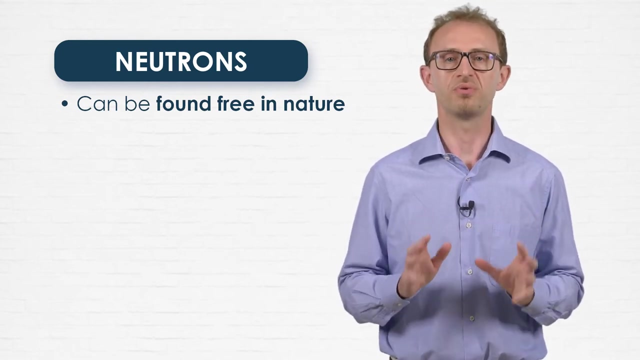 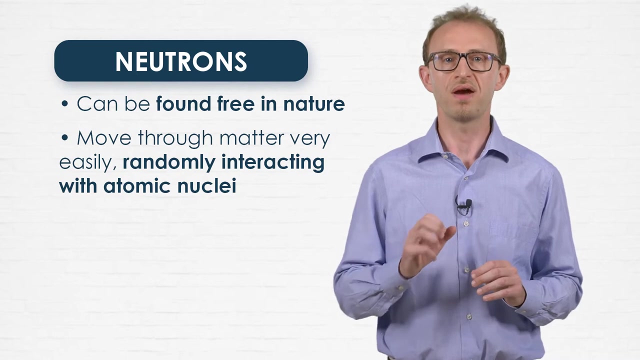 short introduction to neutron detection. Let's start with an experimental evidence. Neutrons, the tiny particles that constitute the atomic nuclei, can often be found free in nature. Not only that, Being neutral, they move through matter very easily, randomly interacting with atomic nuclei through very 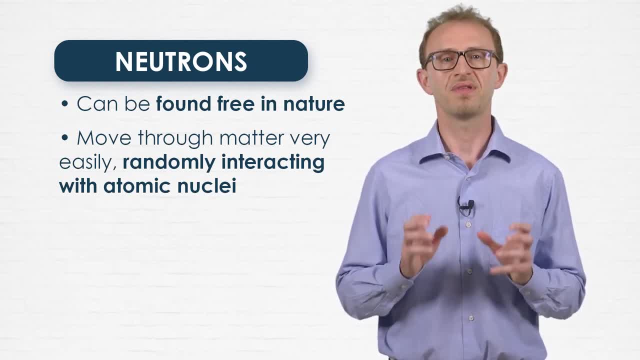 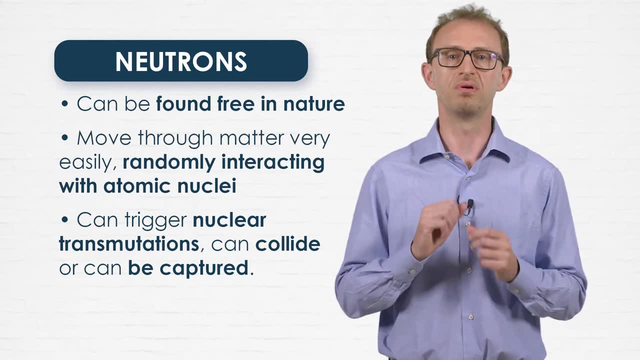 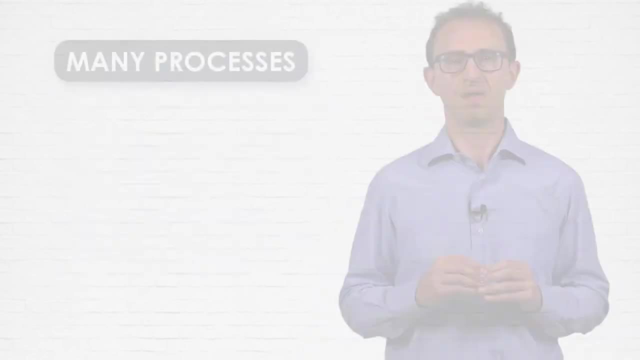 different nuclear reactions. Depending on their kinetic energy, neutrons can trigger nuclear transmutations, can collide like billiard balls or can be captured. But where do free neutrons come from? The answer to this question is not unique, because many different processes 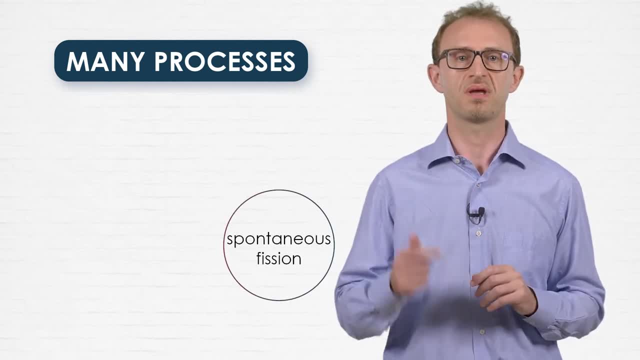 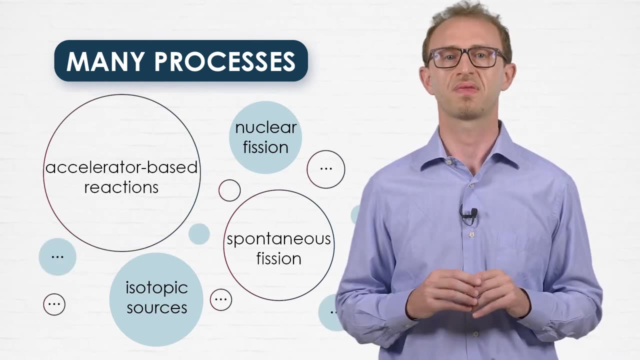 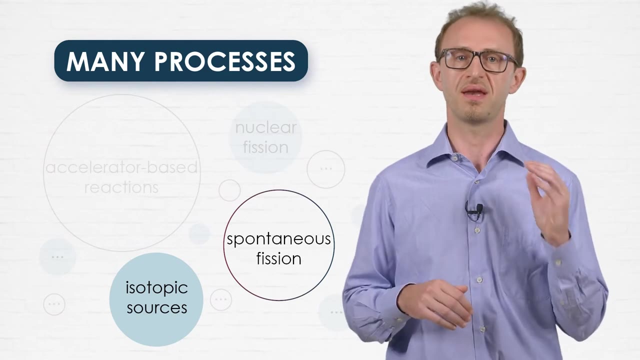 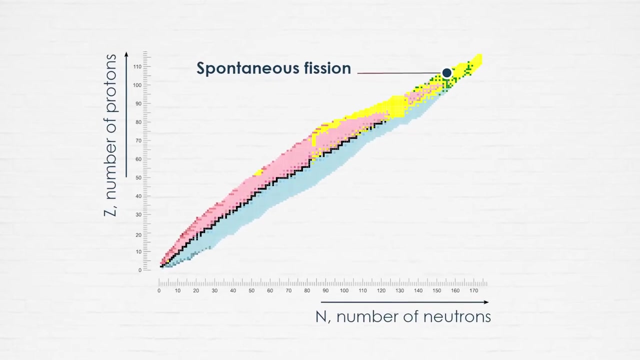 are linked to the emission of neutrons: Spontaneous fission, isotopic sources, nuclear fission, accelerator-based reactions and many others. Let's consider as useful examples just two of them: spontaneous fission and isotopic sources. Spontaneous fission is a decay process that produces, let's say, directly, neutrons, As 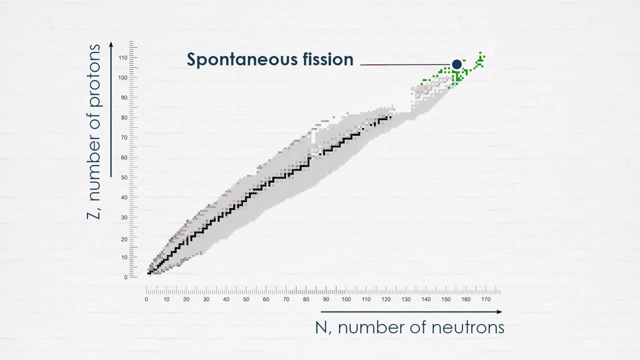 indicated by green regions in the table of neutrons. neutrons are the particles that produce neutrons. In the table of nuclides, the spontaneous fission is typical of some heavy nuclei. as an alternative to other processes In a spontaneous fission, an unstable nucleus. 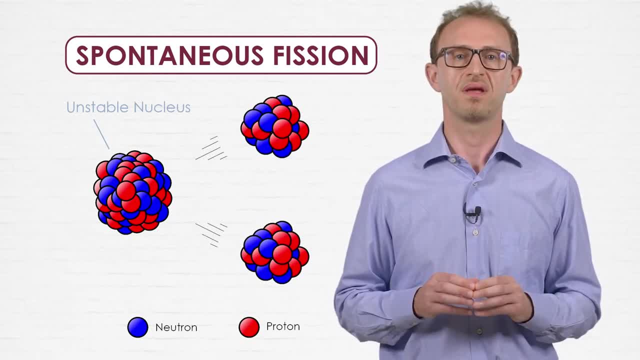 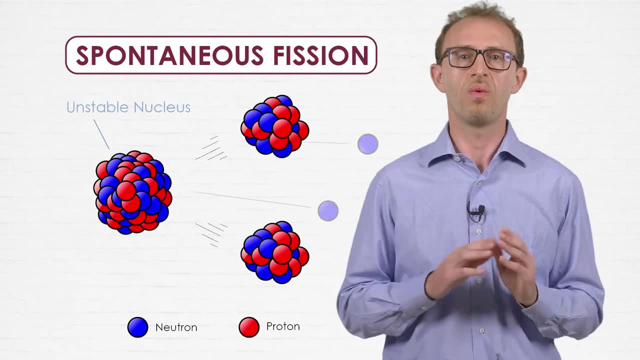 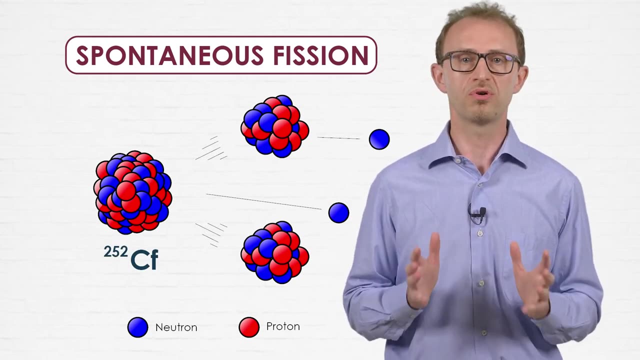 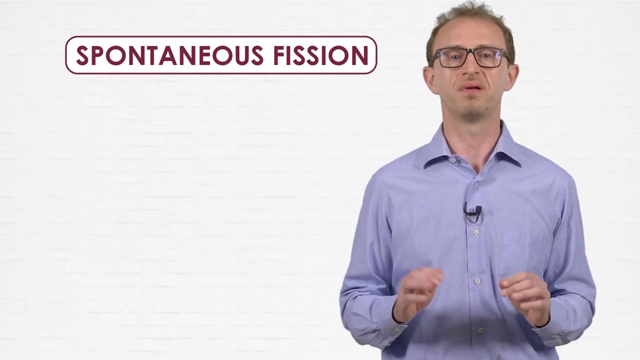 splits into two lighter nuclei. The products are always highly unstable and eject sooner or later one or more neutrons. The leader of this category is Californium-252,, which is the most widely used neutron source from spontaneous fission. Anyway, this is just an example, but it is practically very important to bear in mind. 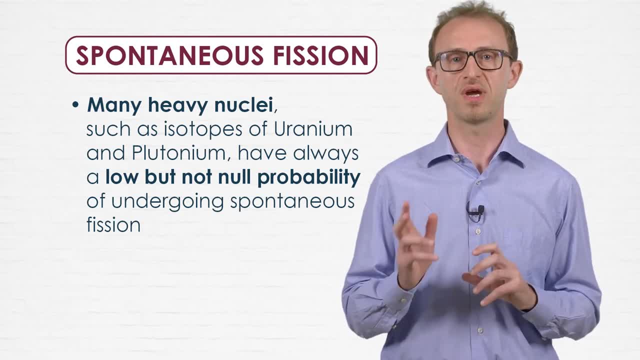 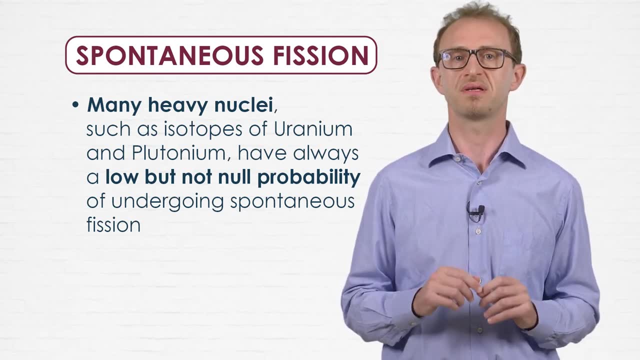 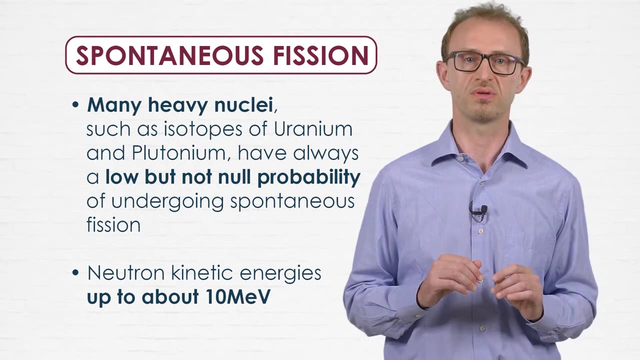 that many heavy nuclei, such as isotopes of uranium and plutonium, have always a low, but not null, probability of undergoing spontaneous fission. In all cases, the typical kinetic energies of fission neutrons are the ones that produce neutrons. The fission neutrons range between tens of keV up to about 10 MeV. 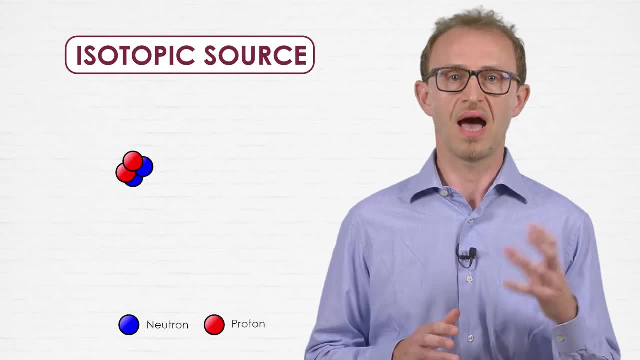 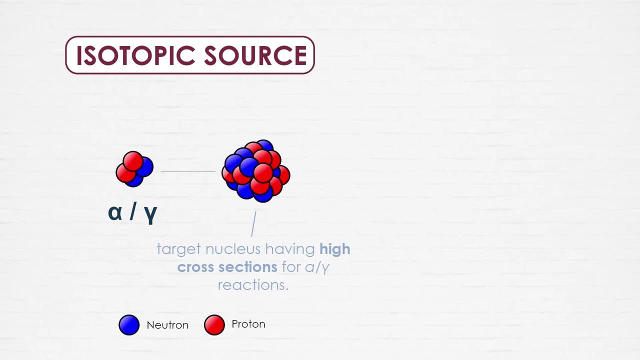 Another way of producing neutrons is to mix alpha and gamma emitters with target nuclei having high cross-sections for alpha-n or gamma-n reactions. In such a coupling, target nuclei react with an alpha or a gamma particles and free neutrons. The typical target nucleus is beryllium, a material that maximizes cross-sections and 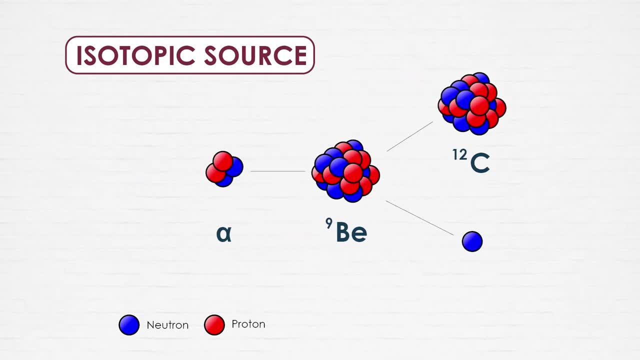 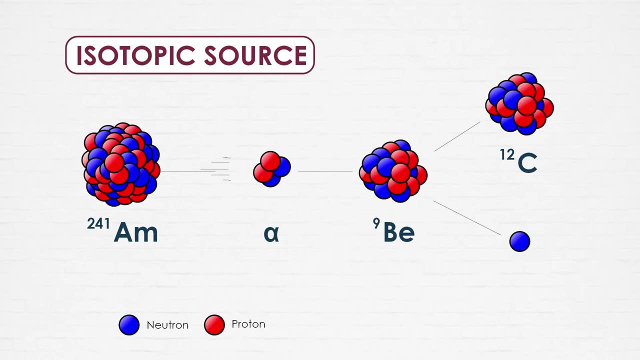 consequently the neutron yield. A good example of isotopic source is the americium-beryllium, an alpha-n source assumed as a reference in the ISO standards. Other examples are plutonium-beryllium, polonium-beryllium, radium-beryllium, curium-beryllium and americium. 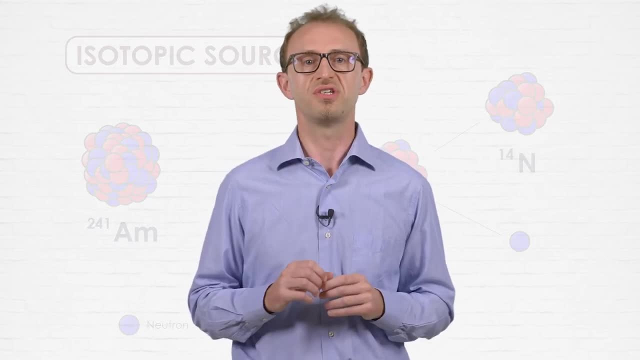 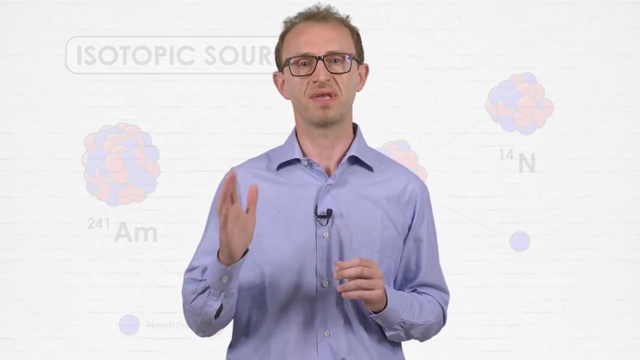 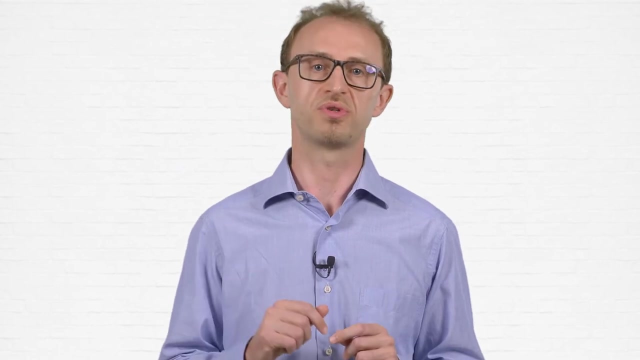 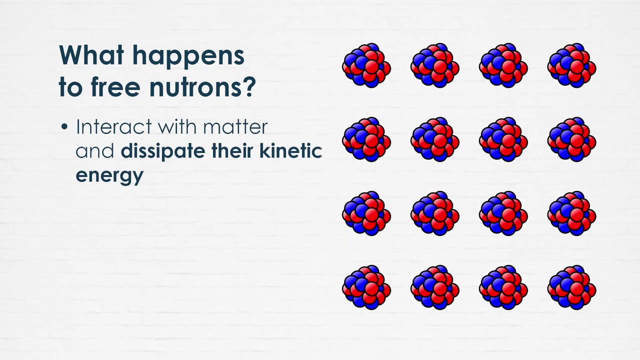 Kinetic energies of neutrons produced by isotopic sources grow from tens of keV up to about 10 MeV. Ok, so far we've had a look at some ways of emitting neutrons. Now what happens to free neutrons? Well, they start interacting with matter via different nuclear reactions. 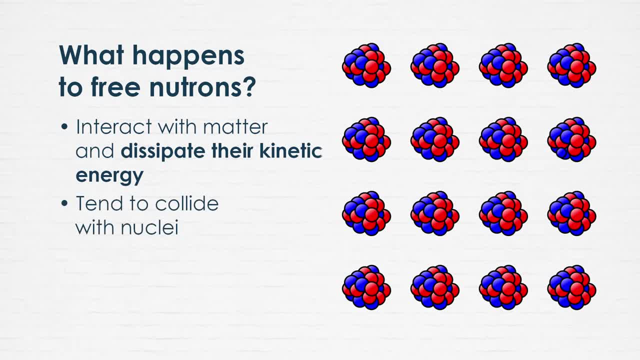 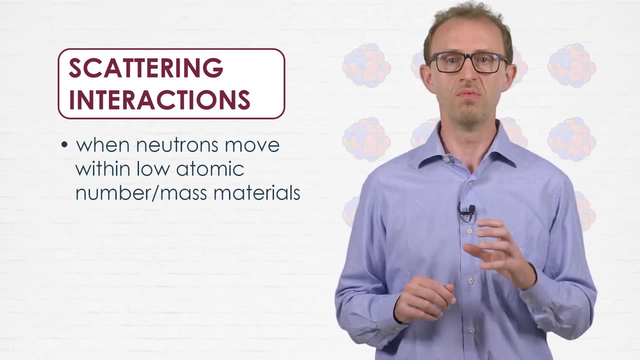 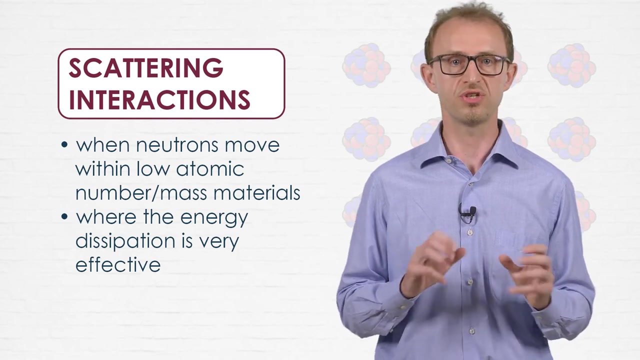 dissipating their neutrons. Being neutral particles, neutrons tend to collide with nuclei by undergoing the so-called scattering interactions. This is especially true when neutrons move within low atomic number materials, where the energy dissipation due to collisions results to be very effective The slowing down process. 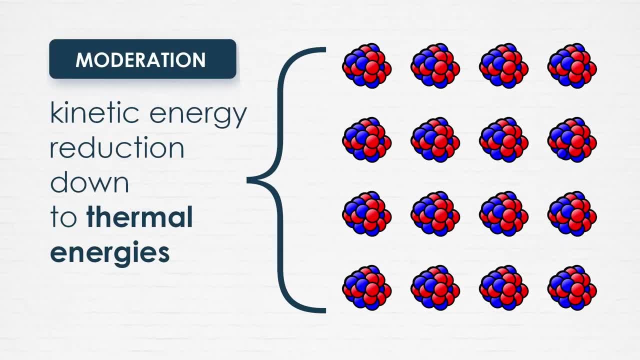 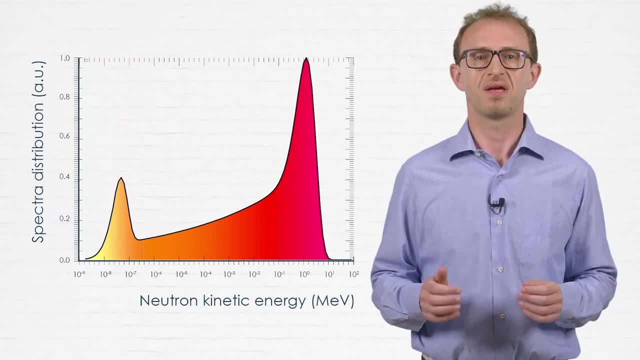 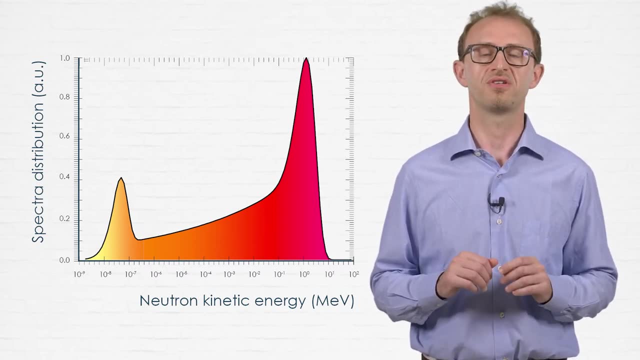 called moderation, ends when neutrons reach the minimum kinetic energy possible, the thermal energy. In real situations, the final effect of such a behavior is the coexistence in the neutron field of all kinetic energy components, from the maximum emission value down to the thermal 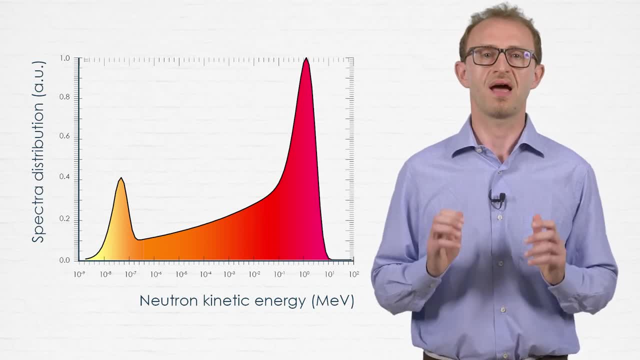 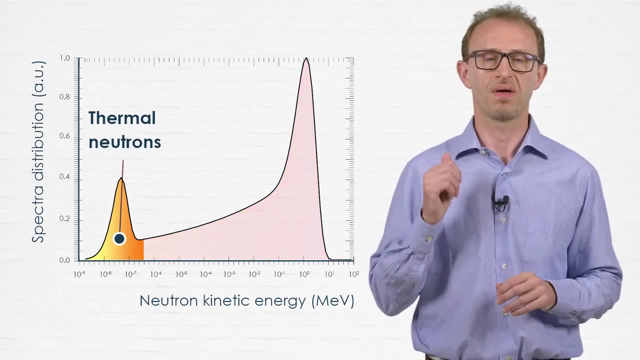 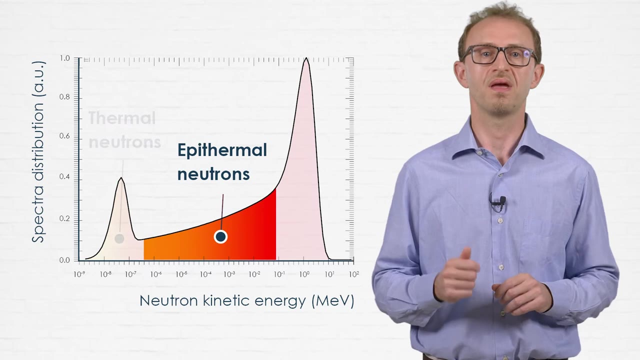 one. For this reason, neutrons up to 20 MeV are conventionally classified according to the maximum emission value of the thermal one. We have thermal neutrons characterized by energy values ranging from 0 to 0.5 eV. epithermal. 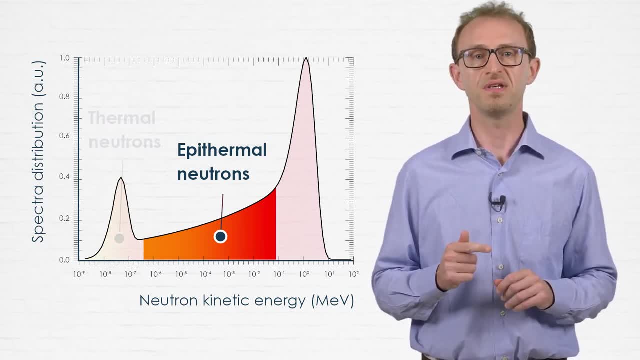 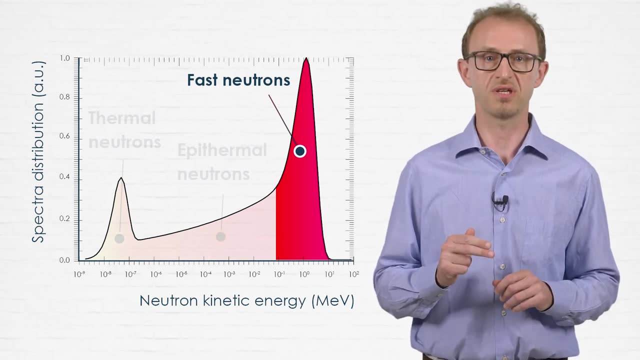 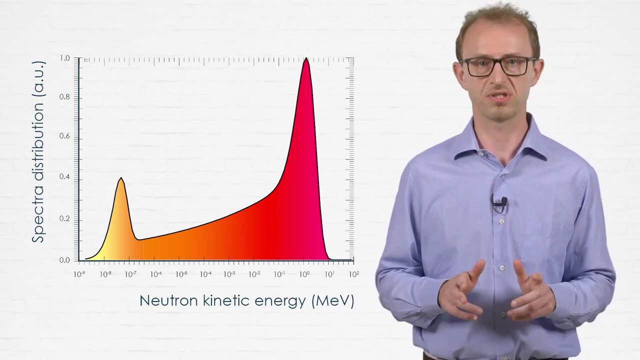 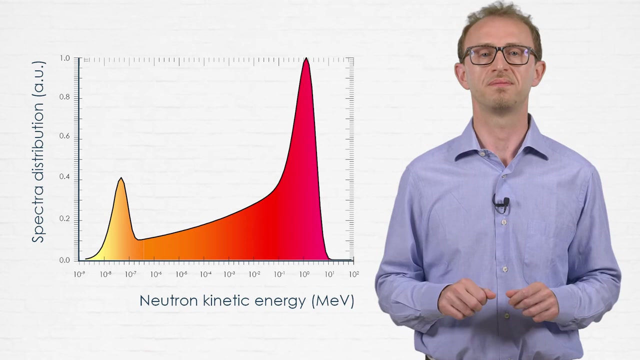 neutrons with energy between 0.5 eV and 100 keV, and fast neutrons with energies higher than 100 keV up to 20 MeV. Each class has its own physical features and processes, features and processes that are exploited also to detect and measure the neutron field. 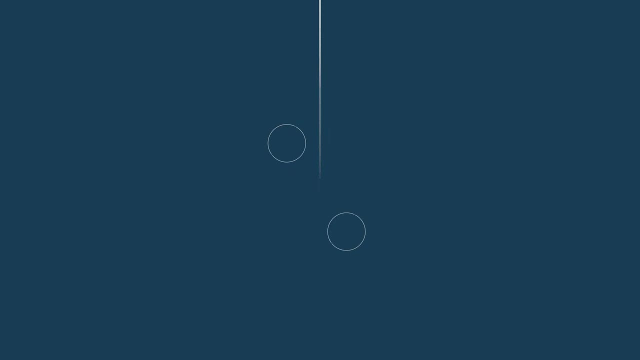 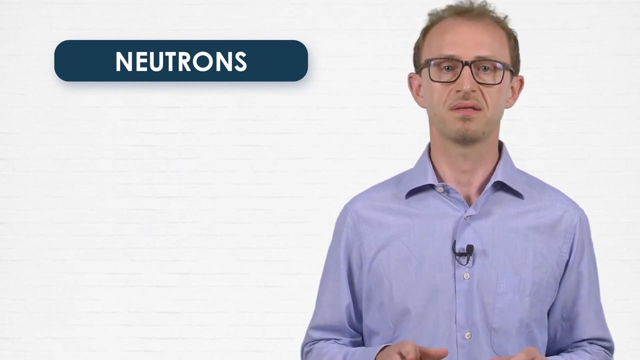 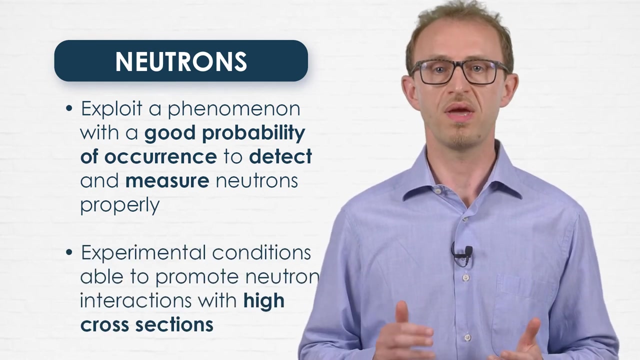 Let's give you some elements about that. First of all, a simple consideration: In order to detect and measure neutrons properly, we need to exploit the phenomenon with a good probability of occurrence. In other words, we have to set up experimental conditions able to promote neutron optimization. 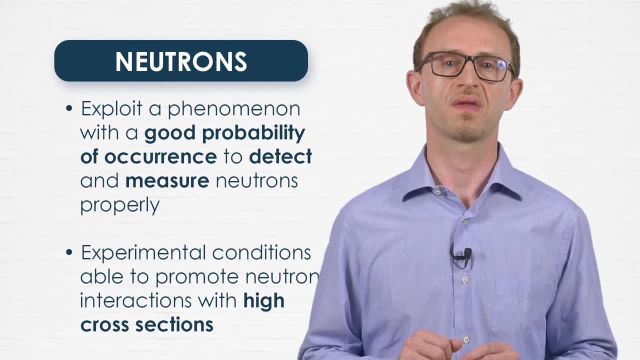 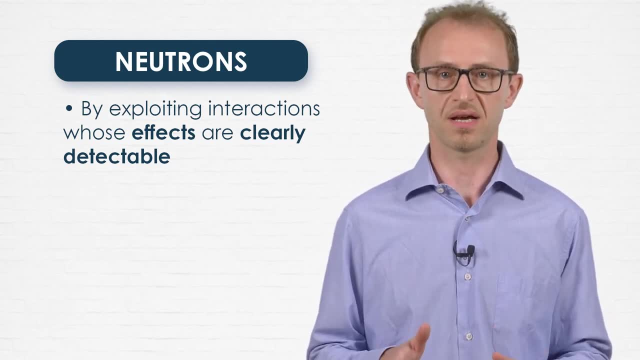 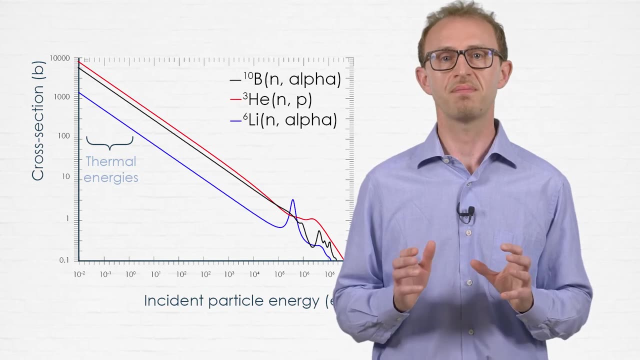 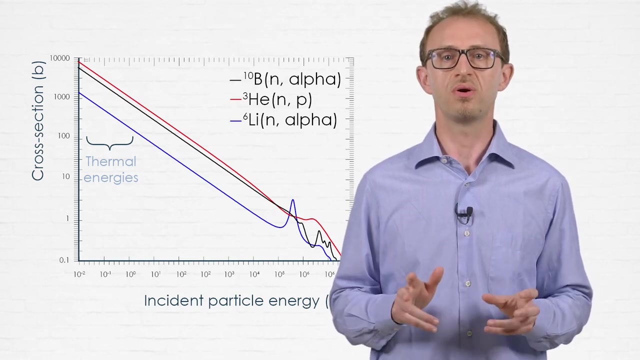 interactions with high cross-sections. Moreover, we must do so by exploiting interactions whose effects are clearly detectable. Well, the experimental evidence shows that these conditions are met by some neutron capture reactions at thermal energies. More specifically, we nowadays know that, at thermal energies, the nuclei Boron-10 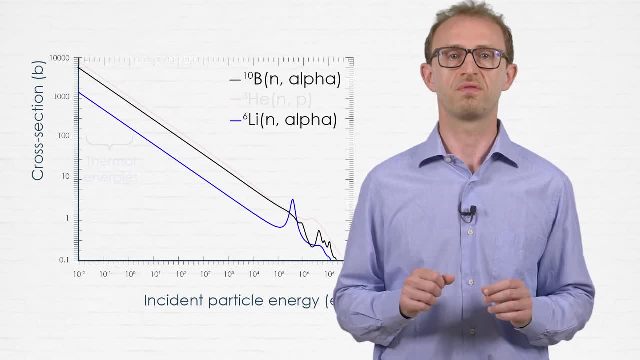 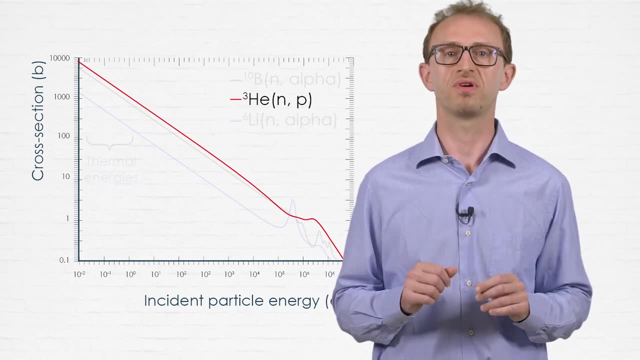 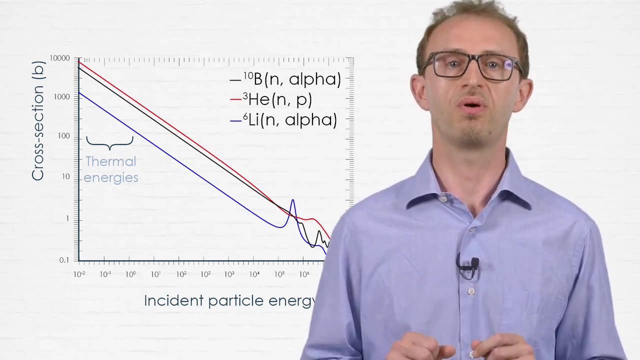 and Lithium-6 have a high cross-section for N-alpha reactions, while the nucleus Helium-3 has a high cross-section for the N-P reaction. This is the reason why thermal neutron detectors are instruments that exploit typically materials containing Boron-10, Lithium-6 or Helium-3.. 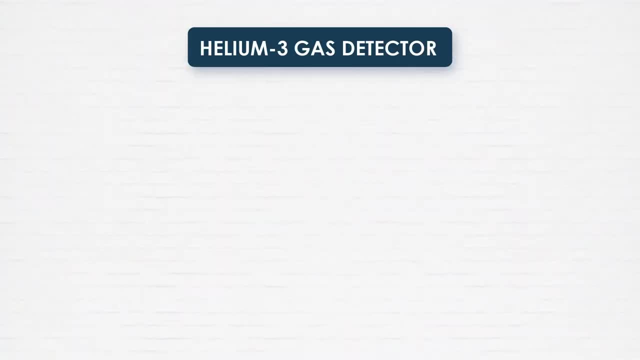 An important example is given by Helium-3 gas detectors. These are cylindrical or spherical chambers filled with Helium gas enriched with Helium-3. By means of electrodes, a proper electric field is set within the chamber. So when a thermal neutron enters the chamber, it is likely to react with the Helium-3 nucleus.